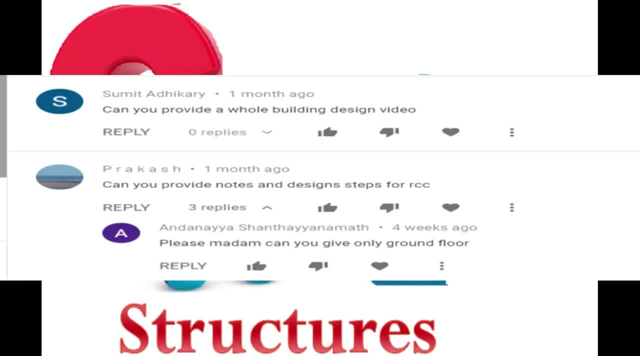 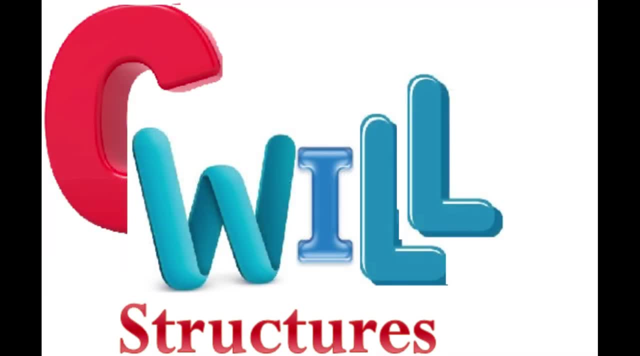 hello friends, welcome to my channel, civil structures. i have received many requests from our subscribers of civil structure family about manual design of g plus one or g plus two. so after giving it a thought and working for some days, i have came up with simple building design which 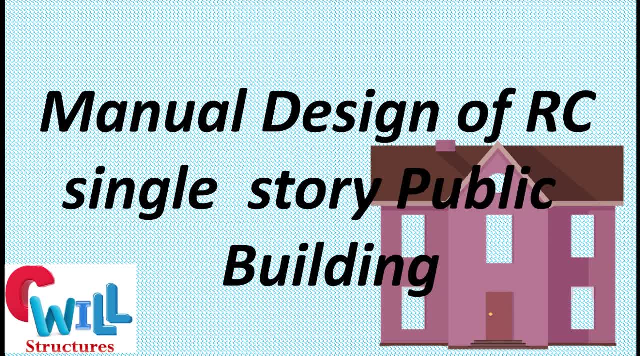 borrows individual structural elements and the basic rcc fundamentals from my previous videos, as we know that the building design actually contains knowledge of individual structural elements, so i will not be explaining the very fundamentals of these structures, as we have already covered it is in past tutorials. however, i will give all possible references through i button. 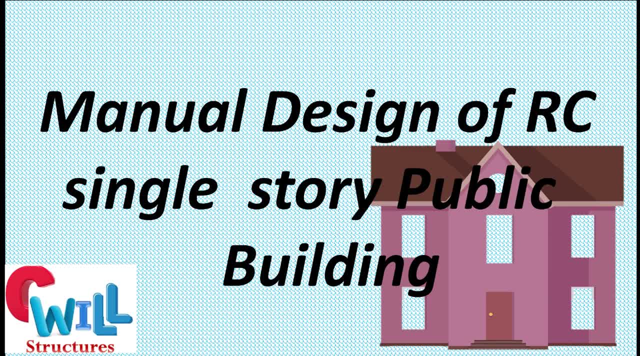 while explaining the design. also, please bear with me for silly mathematical mistakes. i'm sure that you will be able to do those calculations. i hope this video series would help you to understand the simple building design concepts and boost your confidence. for beginners, i would recommend: don't forget to subscribe to my channel and i will see you in the next video. bye, bye. 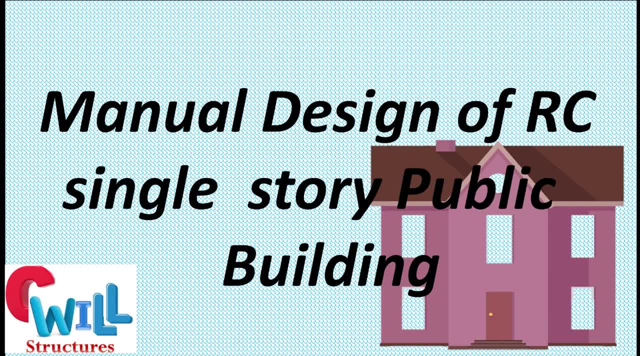 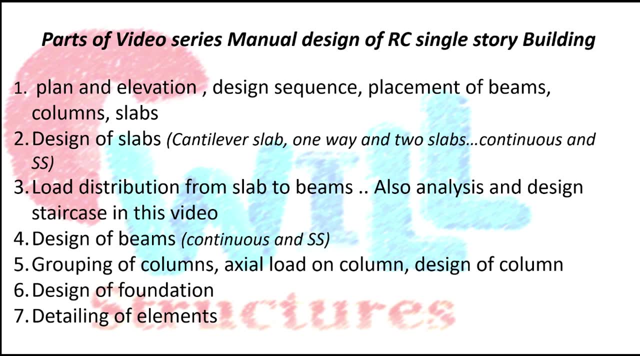 do not skip any video of this series and go through the chronological order these video series. manual design of rc single story public building consists total seven parts and they are: in first part we will discuss the plan and elevation of building. then we'll discuss the design sequence. 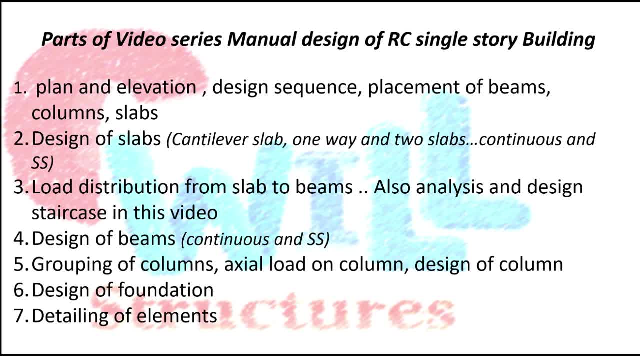 and then the placement of beams, columns and slabs. in second part we will learn how to design the slab, whether it is cantilever slab, one way, continuous or simply supported, or maybe it is simply supported slab. in third video we'll discuss the load distribution from slab to beams. we will 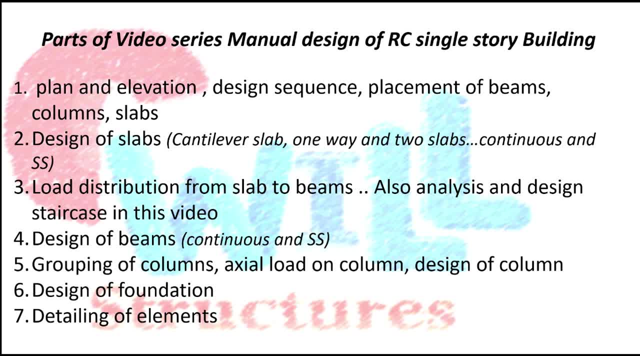 also analyze and design staircase in this video. in fourth part, we'll design the beams, whether it is continuous beam or simply supported beam. in part five, we design the columns. definitely we'll do the grouping of columns, whether it is actually loaded, whether it is actually loaded plus uni-axial. 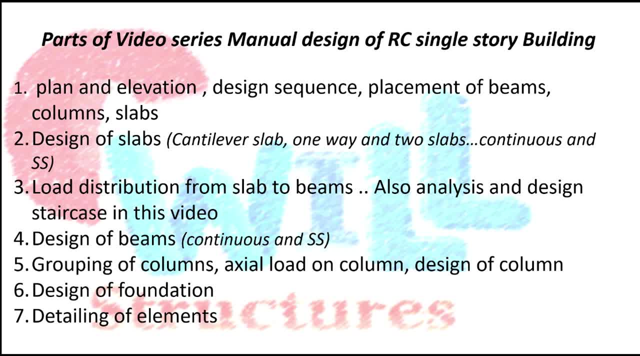 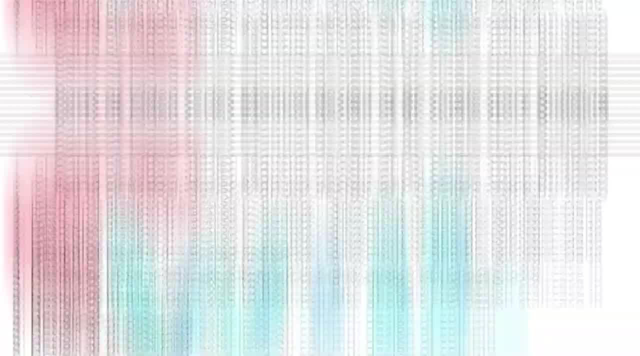 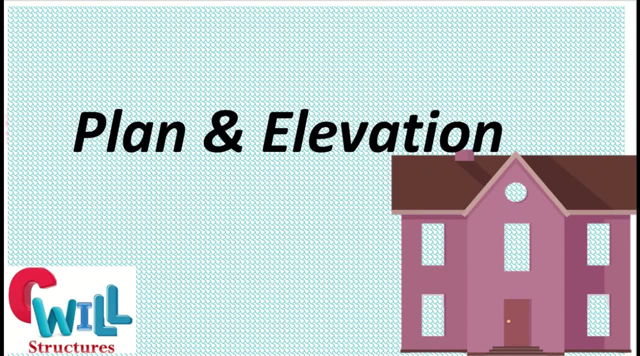 or a3, or it is actually loaded plus biaxial column. in sixth part we'll design foundation and in the third part we'll explain you the detailing of this particular elements. okay, so let's start part one for the manual design of rc single story public building. okay, now let's see first plan and 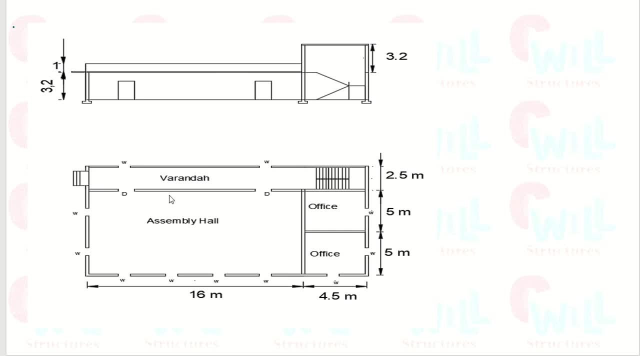 elevation of the building. you can see this particular drawing. here is the plan of building and here is the elevation of building. i have chosen this building for design of the manual structure. okay, now let's first understand this particular plan of the building. first tell you: here is public building. now let's see the plan of a building. this plan is dividing. 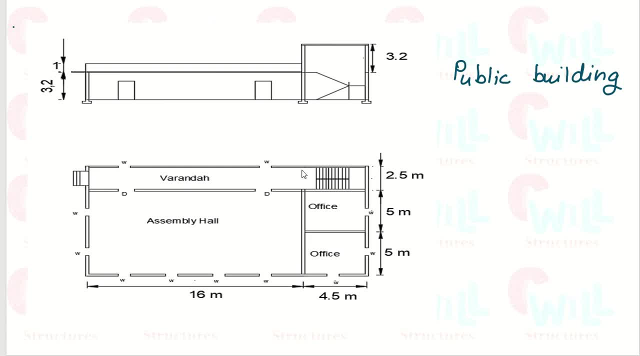 in different areas. there is assembly hall- this particular portion is veranda, and here there are two offices and one stack s. is there okay? i mean, if you see, the length of structure is almost 20.5. let me just draw here, okay. so this length is 20.5 meter, in where 16 meter by 10 meter is. 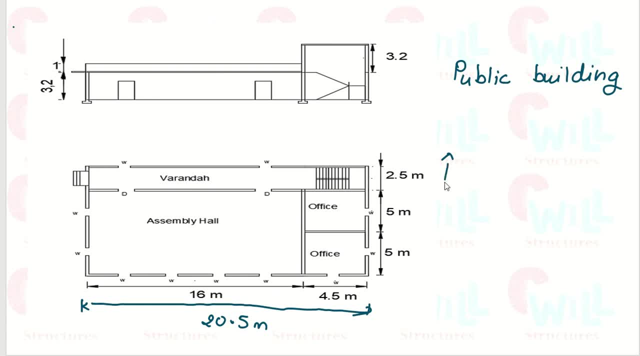 actually measuring the height dimensions, sorry, the height distribution, the high-uth애. so we are taking this空 part to be measure so a long милли hall. we are taking here center to center distance for the wider direction when it is 12.5 meter if you see in the elevation we can understand. 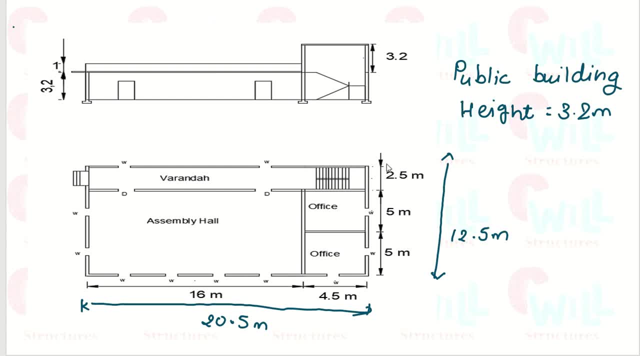 only not for the throughout 12.5 meter. so here for the particular 2.5 meter is only extended up to one story. okay, so you can see here in the elevation. the another story is also with the 3.2 meter height and we are having one meter parapet wall with the external periphery of the. 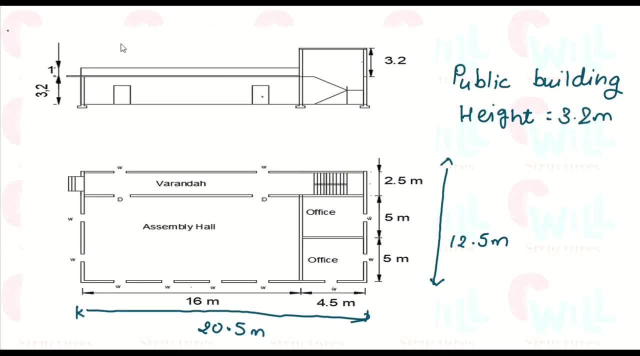 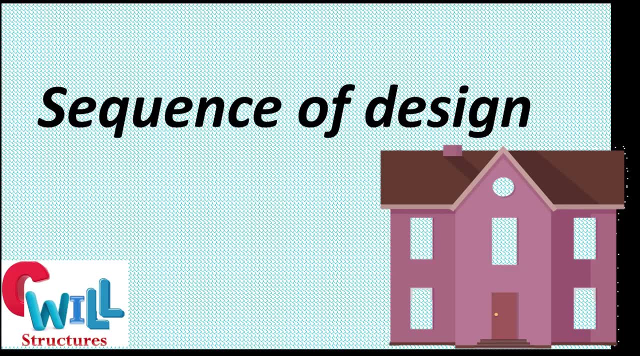 building. you can see here a chhaja which is extending from the top roof, and we can design this as a cantilever slab. now let's see the procedure step for the design of building. so, after understanding the plan and elevation of building, next step is we have to do the placement. 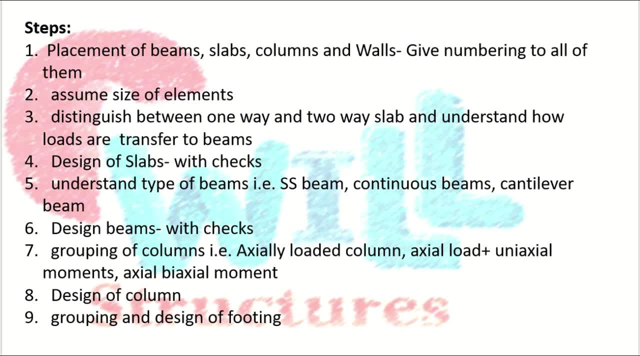 of the beams, slabs, columns and box, with the numbering of all of the elements. then we have to assume the size, distinguish between one-way slab and two-way slab and understand how the loads are transferred to the beams. next is start with the designing of slab, with all checks, of course. 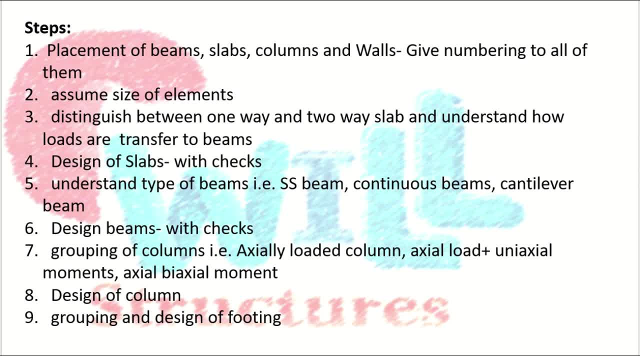 with the detailing drawing. then we have to understand the type of beam, whether it is simply supported beam, it is continuous beam or it is cantilever beam. we have to design the beam with all necessary checks and with the detailing drawing, the grouping of column, and understand whether it is actually loaded- axial loaded plus uniaxial moment or maybe axial loaded. 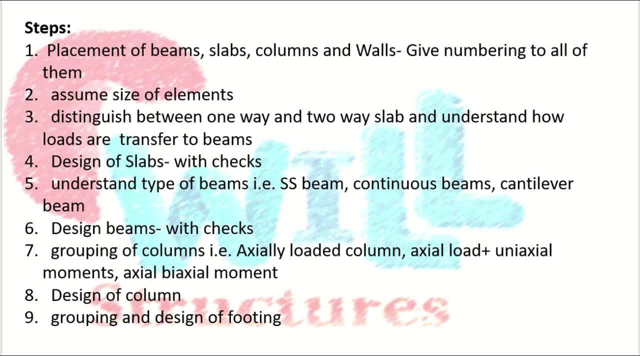 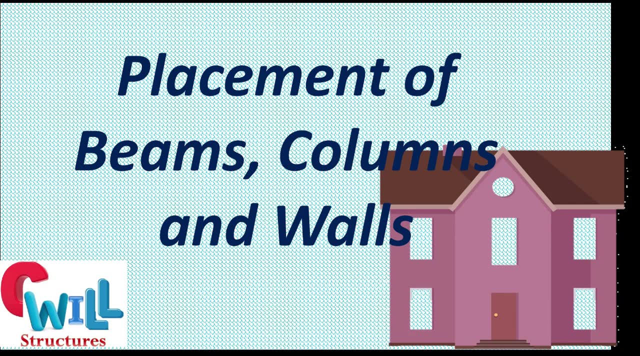 plus by actually and finally, we have to do the design of columns and after designing of column, we have to proceed with the grouping of footing and designing of footings. so we'll do our designing in. the next step is the placement of the beam column and the walls in this particular plan. okay, now 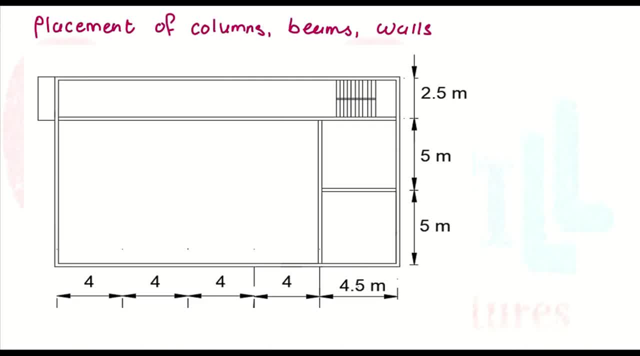 let's first place the columns in this particular plan. of course we will start with the corners. before that we have to choose the size of columns. we can take square column or we can even take rectangular column. the minimum size of column, if we are using m25, it should be 9 inches by 9 inches. 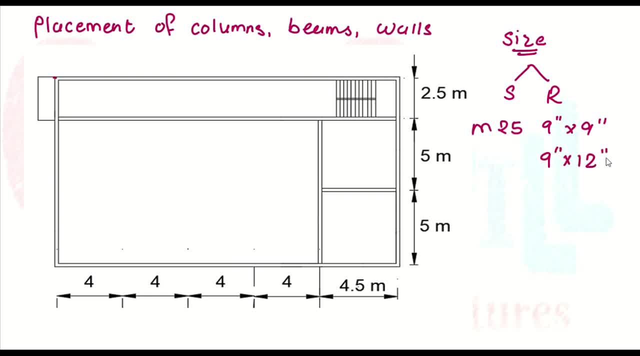 if we are using rectangle column, it should be 9 by 12 inches. let's not talk in terms of inches if we are talking in terms of mm, the minimum size for the column. if we are using square column, it should be 20, 230 by 230 mm and if we are using rectangular column, it is 230 by 450 mm. for now, 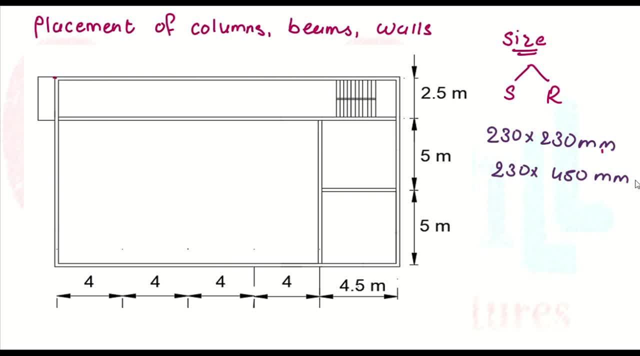 i am assuming rectangular column size is 230 by 450 mm for the particular building. okay, let's see the placement. initially, we should place our columns at the corners of the building. okay, so i am providing rectangular column at the four corners. we should not take more than five meters. 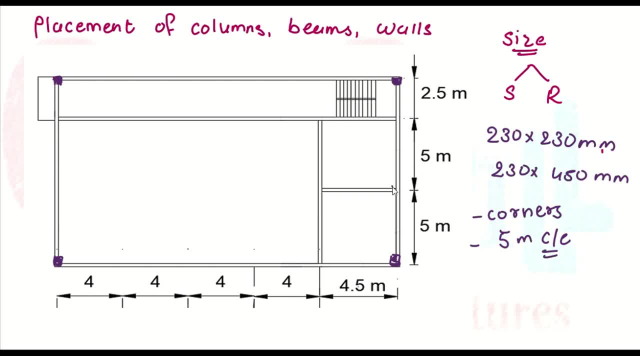 distance between two columns. okay, so i can provide my columns. you can see here, the distance between two columns here is five meter, so i'm not taking more than five meter. we have to take columns the periphery of the stack cabin, so i'm providing here the periphery of the stack cabin, you can. 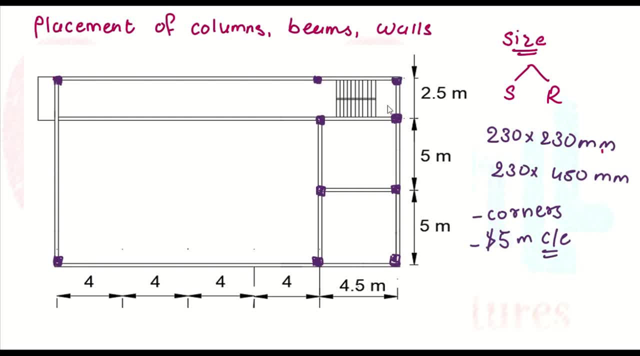 see here. okay, this four column is at the corner of the stack cabins. okay, next now, what about the interior ones? interior columns: now we know that here is the assembly hall and here is the verandah. the width of the veranda is only 2.5 meter, so we could not provide within the veranda. we just 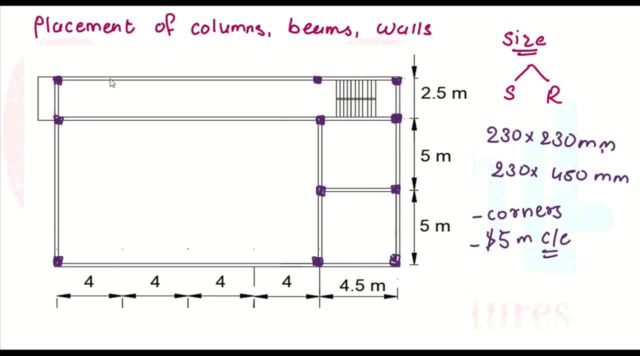 along the periphery of the veranda. and here is this for onellow problems. here we have two columns. we should not keep the distance more than 5 meters. Okay, so I am taking only 4 meter. Also, we cannot provide columns within the assembly hall, otherwise it will be obstructions. So we can. 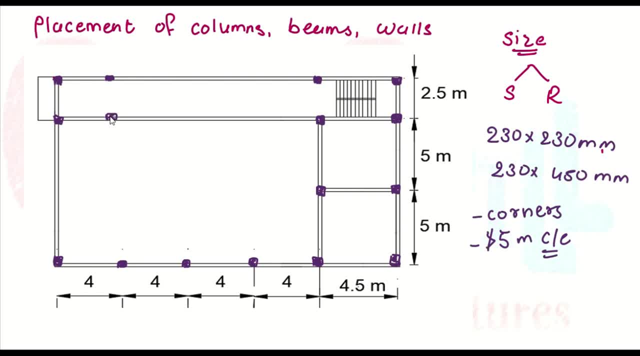 provide at the periphery of the assembly hall, and I am keeping. the distance between two columns are 4 meter. The alignment of the columns should be uniform, otherwise it will be difficult to cast the columns. Also, it will be difficult for the casting of beams and the walls. Okay, so here is. 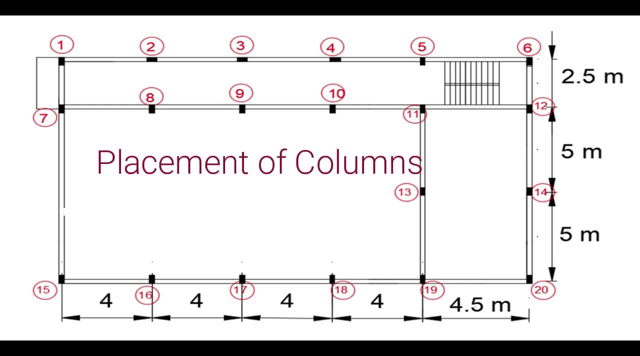 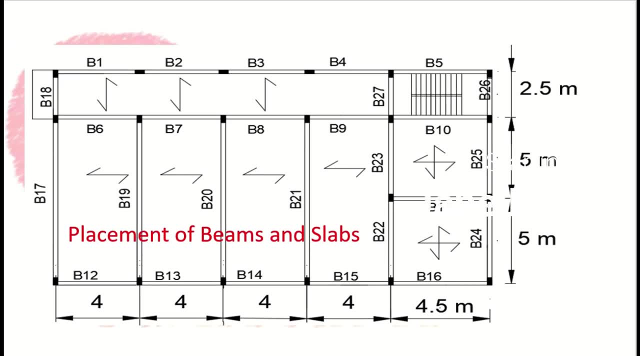 total number of columns we have provided in our particular plan. Now let's talk about the placement of the beams. We can just connect the columns and we can provide our primary beams. As you can see, we have total 25 number of beams here. All are primary beams as they are supported with columns. 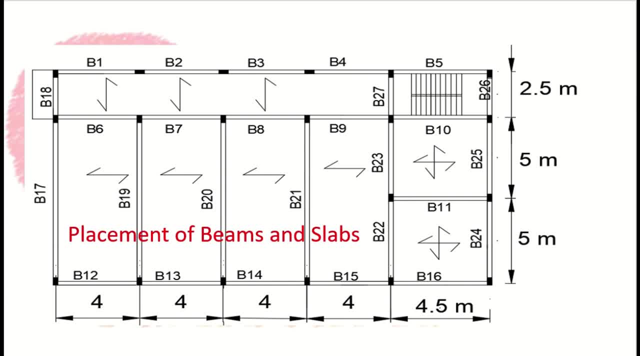 at both ends. Now see here Which beams are continuous Beam: B1, B2, B3, B4 and B5. They act as a continuous beam Also here: B6, B7, B8, B9 and B10. 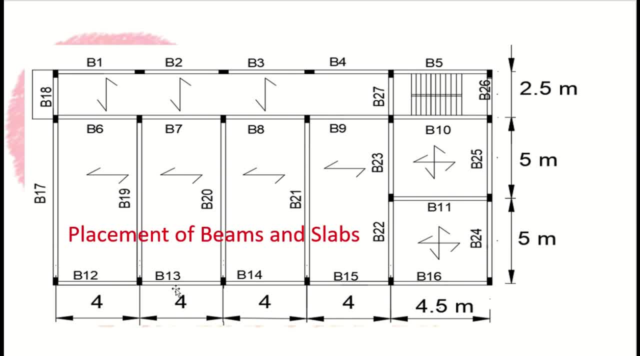 They are also continuous beam. Okay, and also this: B12, B13, B14, B15 and B16.. These also act as a continuous beam. All these continuous beams consist 5 span. The other continuous beams are which are having 2 span, and they are B1, B2, B3, B4 and B5.. So these are continuous beams, So we can just. 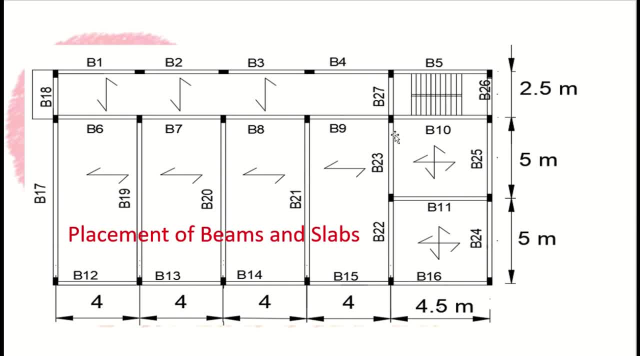 connect B17 and B18.. B22, B23 and B24 and B25.. And the remaining ones, B11, B26 and B27. they are simply supported beams, where my B27 and B26 are the beams at the end of landing of staircase B26. 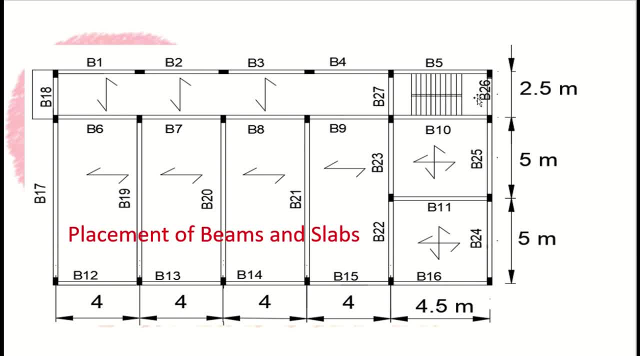 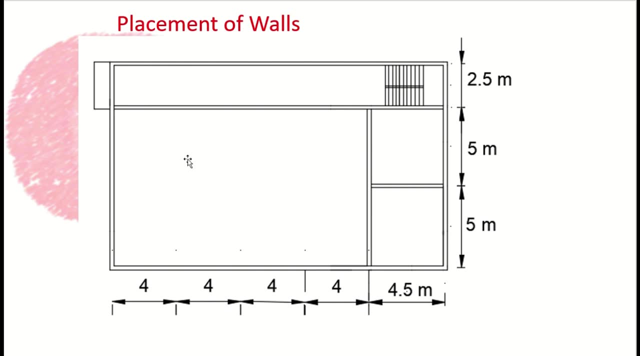 is at mid landing level beam. It is at the mid level of the story height. During the design of the beams- we will discuss this in detail Now- below the beams we generally placed walls. but we can not construct the wall in between the assembly hall, otherwise it will be obstruction. 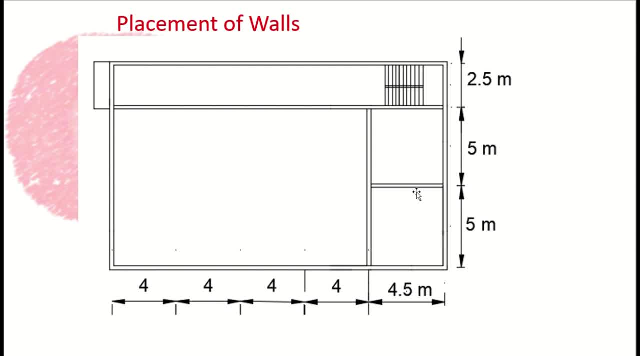 So we provide the walls at the periphery of building. Also, let's separate the each and every part of the building, such as veranda, assembly hall and two offices. Also, let's provide the wall extended story at the periphery of staircase, And here is a diagram for the walls. Now let's 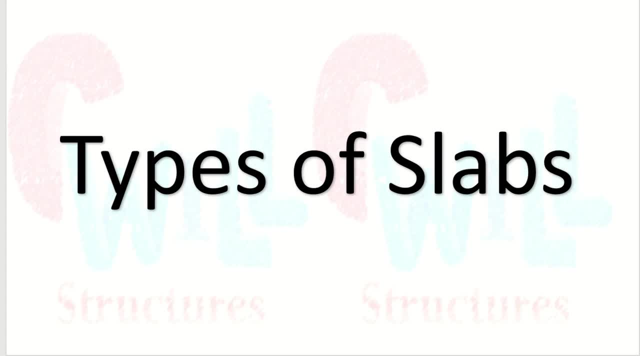 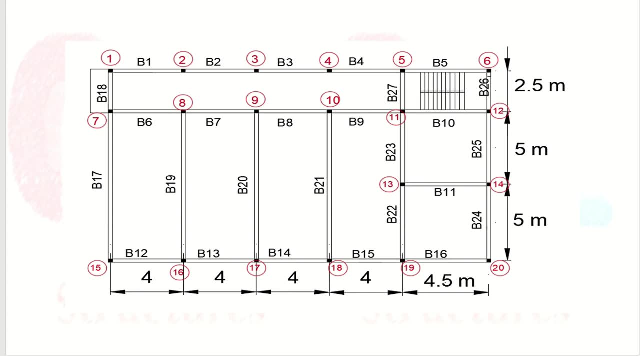 discuss the types of slabs are in the particular building. Okay, we can see here this, this, this: these are the number of slabs here. Now we have to decide which are: the cantilever slab, one-way slab and two-way slab. So how can we understand? Okay, as we already discussed, here is a type: chhajja type. 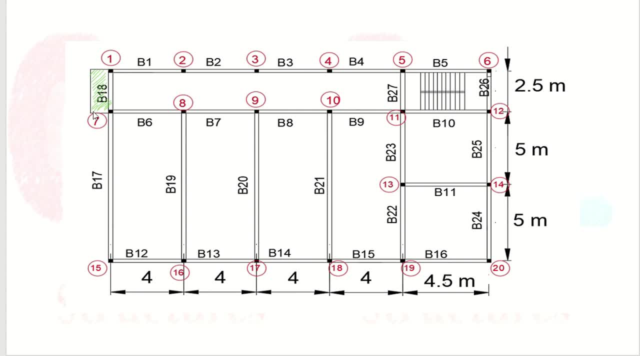 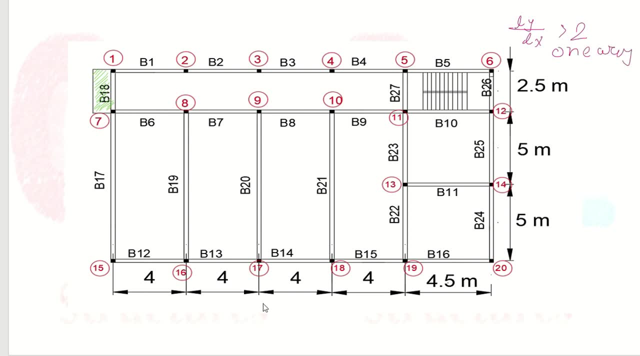 So this is my cantilever slab. How can we discuss our one-way slab? If ly by lx is more than two, then it will be one-way slab, right Okay? and if my ly by lx is less than two, then it will be one-way slab. 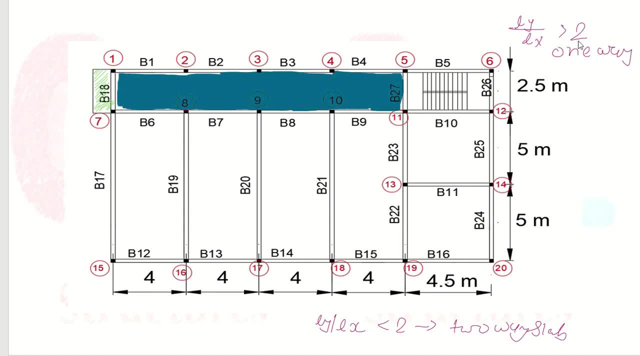 Okay about this particular slab where ly by lx ratio is more than two. Let's calculate where ly is 16 meter divided by the shortest span is 2.5 meter and here the ratio is 6.4.. So we can consider this whole slab as one-way slab. How to show one-way slab in particular? plan with that. 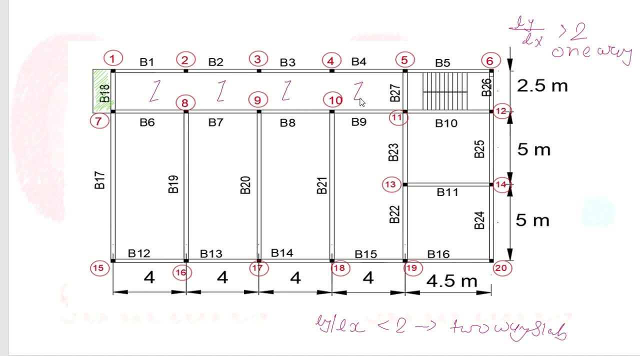 direction of main reinforcement. Okay, and we know that main reinforcement in one-way slab is along the shortest span. Okay. so if this is my shortest span, here is the direction of main reinforcement and here is a sign to show the one-way slab in Now. 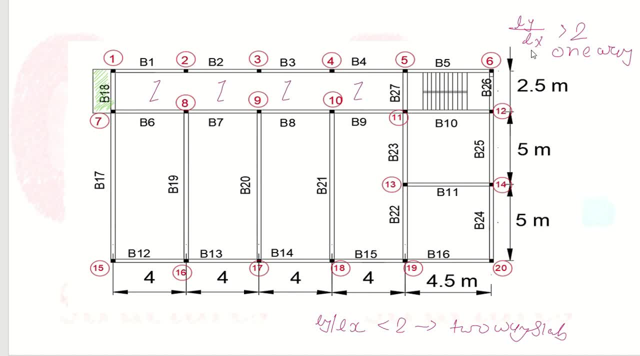 let's talk about all the slabs: 1,, 2,, 3 and 4.. Before that, let me give the nomenclature of the slabs. Okay, so let me give the nomenclature for the cantilever slab, as in S1.. So let me write here. 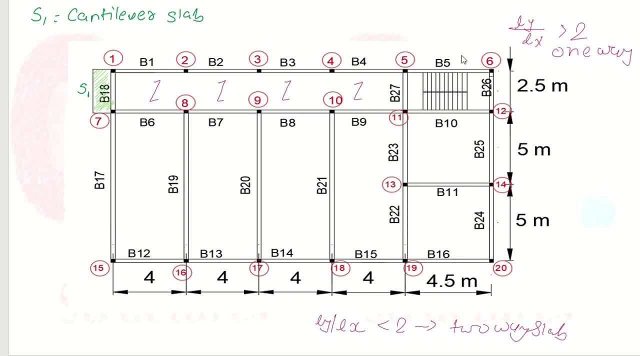 S1 is cantilever slab. Okay, now, S2 is this particular whole slab which is having size 16 by 2.5 meter. I'm giving the name here: it is S2.. Okay, now Here, S1,, 2,, 3 and 4, I'm talking about all this, this four slabs. Okay, well, the size are same, the size. 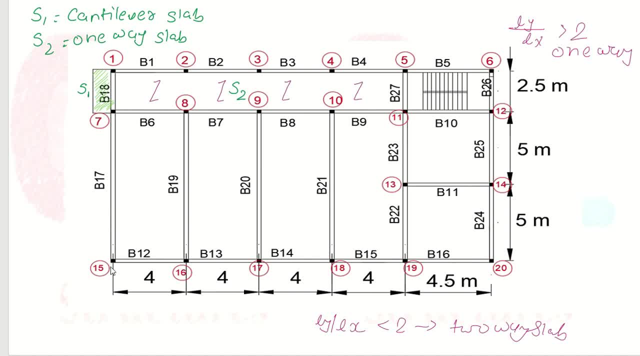 for longitudinal longer span is 10 meter and the shortest span is 4 meter. Again, let's calculateектор situation. Let's calculate ny-lx بت: 10 meter. 4 is 2.5, again it is more than 2, so these four slabs are also one-way slab. and here my direction. 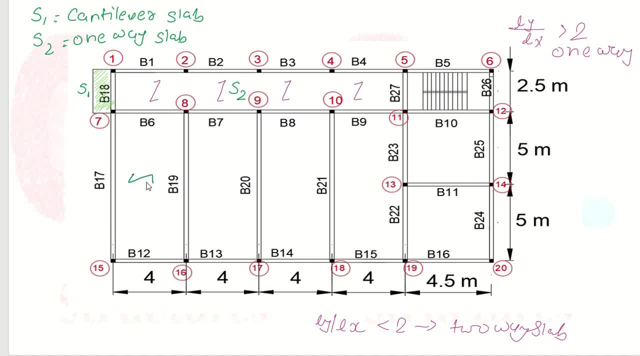 of main reinforcement is along shorter span. so this is my direction of main reinforcement, right? okay, so these are the one-way slab, and the dimension of this slab are different than the s2 slab, so i'm just giving the different name: it is s3. but these all, these all four slabs are: 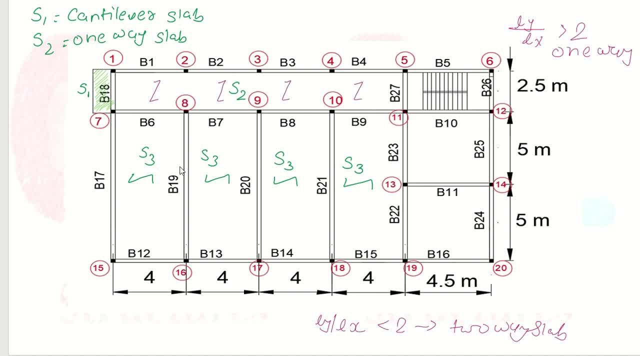 having same size. so i'm giving the same number because design of these slabs are similar. okay, now the other slabs. i'm talking about these two slabs which are having the size: larger span is 5 meter and the shortest shorter one is 4.5 meter. now let's calculate again: ly by lx ratio it is. 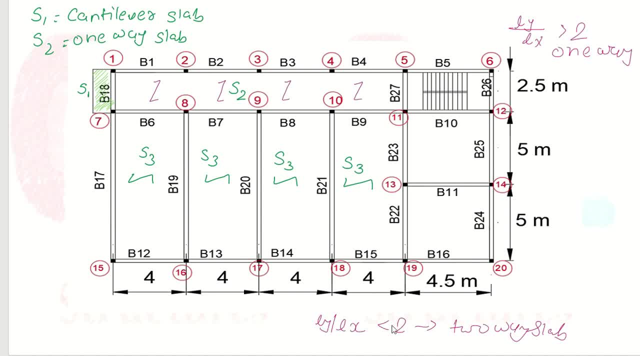 1.11 and it is fall in particular this category. so here, ly by lx ratio is 1.1 and we can consider this: two slabs are two-way slabs. okay, and how to show the two-way slabs with the sign convention like this? why? because here the in two-way slab, the main reinforcement will be in both direction. 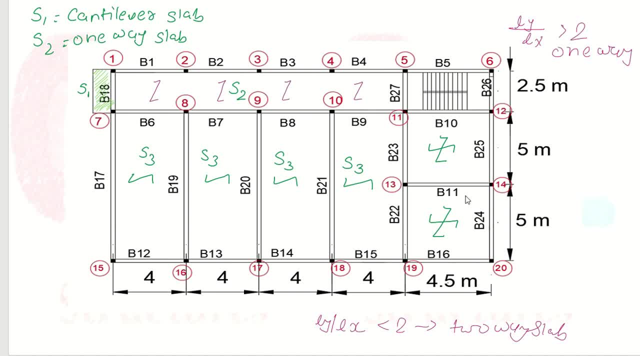 again, these two slabs are having same size and the design will be similar. so i'm just giving the 2.5 meter and it is fall in particular this category. so here the lx ratio is 1.1 and we can number s4- s4. both are having same name. okay, now the remaining slab, that is one slab which is 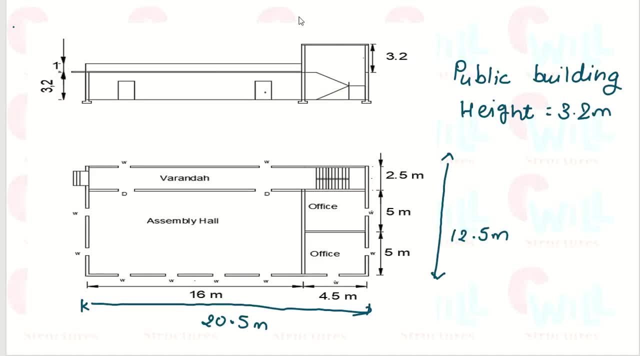 remaining, which we already discussed, for the elevation of this building. i already discussed this. that is one story, but we can say that is one extended. that is one extended story on particular staircase area. okay, so my stack cabin having the slab, but at the 6.4 meter height. here there is not full slab for the stack cabin at 6.4. 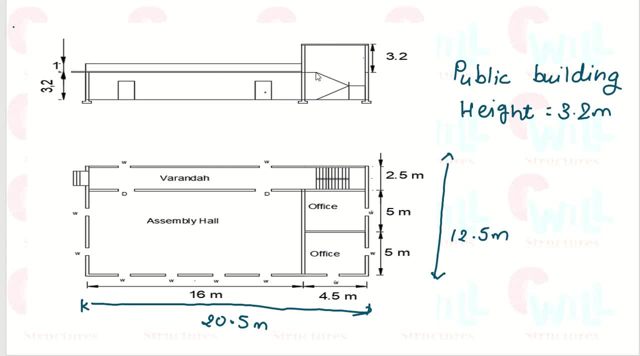 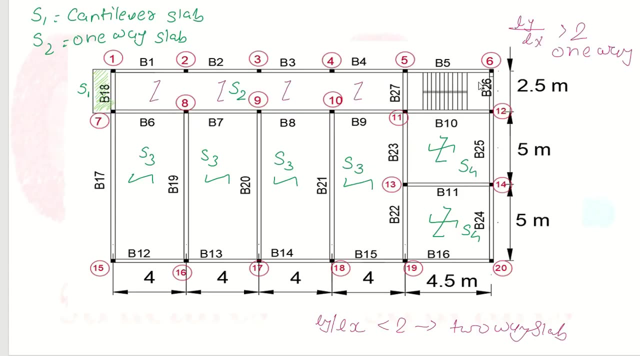 meter height at the first story level. okay, we don't have slab here. you can see in the elevation and we have slab here in this particular elevation. now we have to consider what is the type of this particular stack as cabin slab and what is the size of the stack as cabin. it is the same as 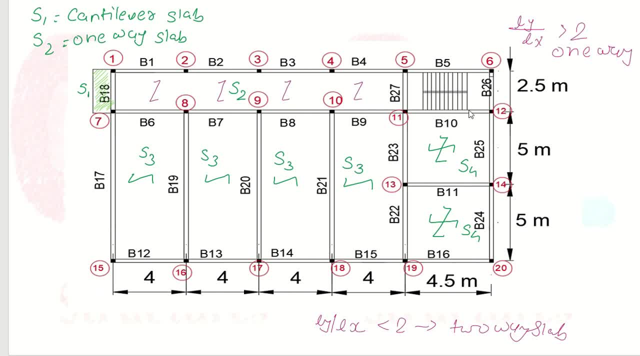 you can see, for the stack cabin at the ground story level and the size is longitudinal. sorry, the largest span is 4.5 meter and the shortest span is 2.5 meter. so if i calculate ly by lx ratio it is less than 2. so 4.5 divide by 2.5 it is 1.8. it fall in this particular category which 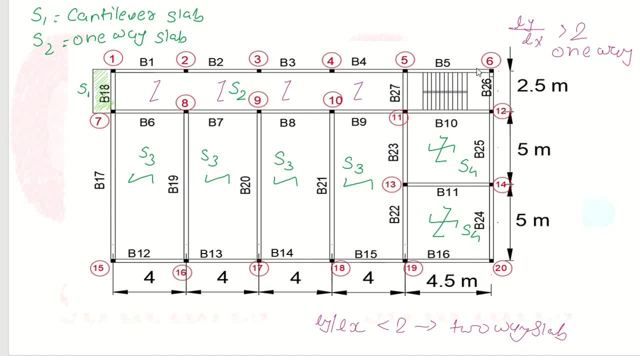 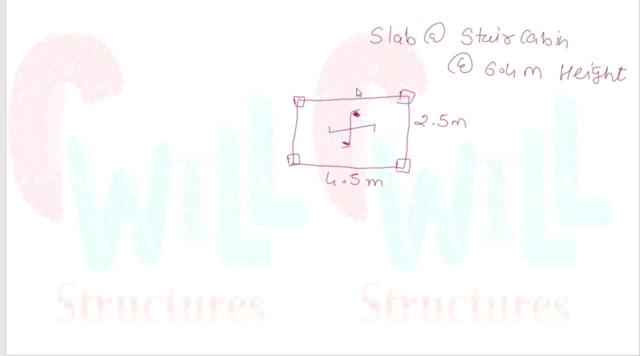 is two-way slab so i can consider this particular slab is okay. so you can see, here i'm showing the particular slab of stack cabin at 6.4 meter height and it is two-way slab. giving the number. it is slab s5, so you just remember that s5 slab. 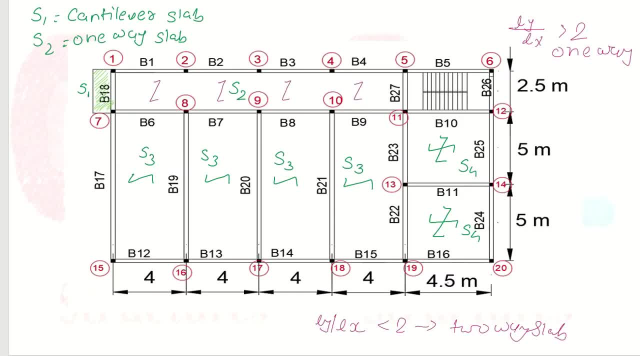 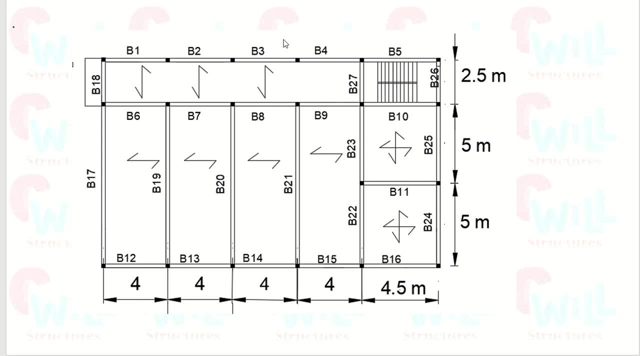 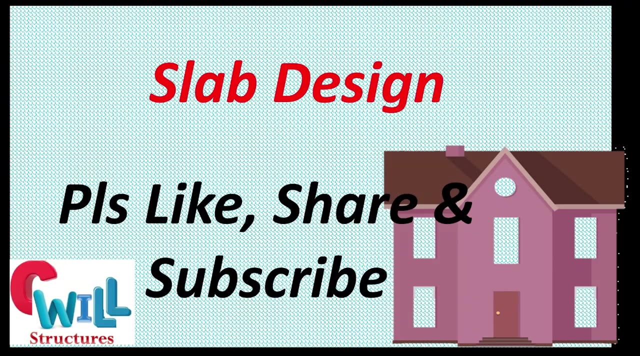 is stack as cabin slab. let's see the complete diagram of one-way slab and two-way slab. so here is a complete diagram, all this slab, beams and columns, including the stack. as in next video of this series, we will discuss how to design the different types of slabs.